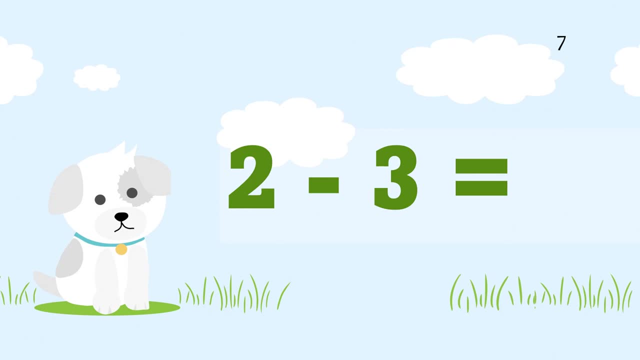 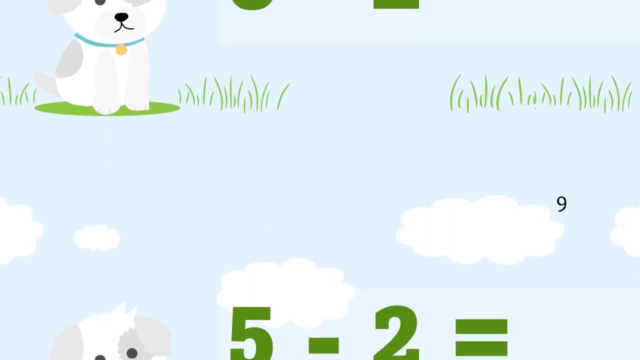 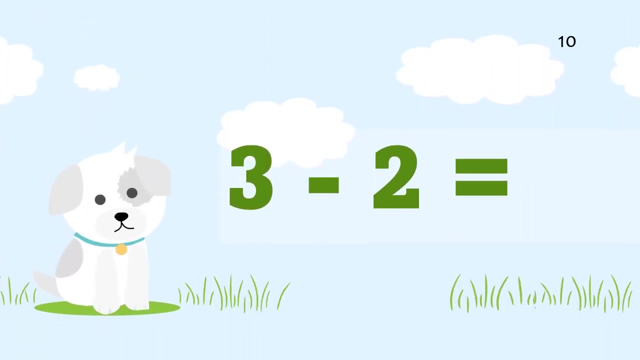 Add a little bit of salt and pepper and mix it. Add 2 tablespoons of cooking oil. Add 2 tablespoons of sugar. Add a little bit of salt and pepper. Add 1 tablespoon of soy sauce. Add 2 tablespoons of cooking oil. 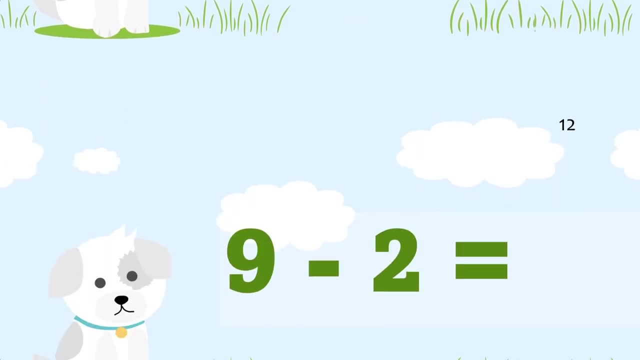 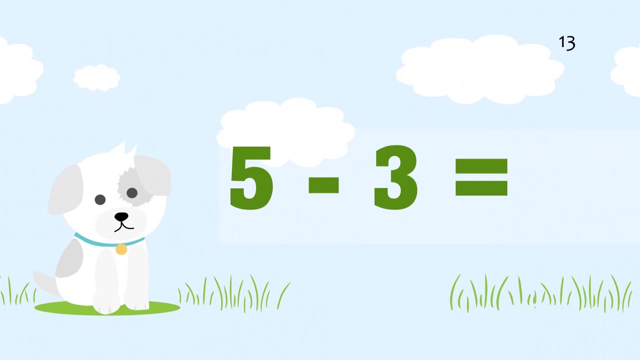 Add 1 tablespoon of brown sugar. Add some kelp and add some soy sauce. Add 2 tablespoons of dark soy sauce. While it's boiling, add the Sieopic. went online. As soon as the soup starts to boil, add two tablespoons of thick sauce. 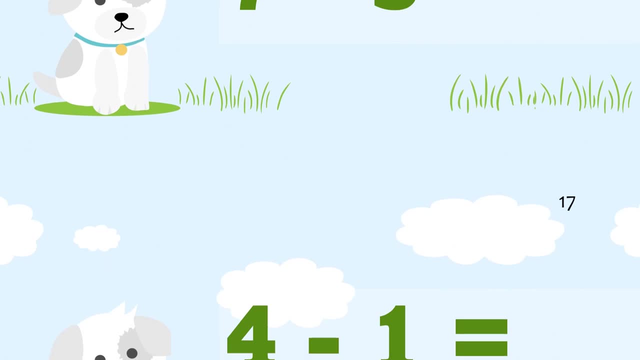 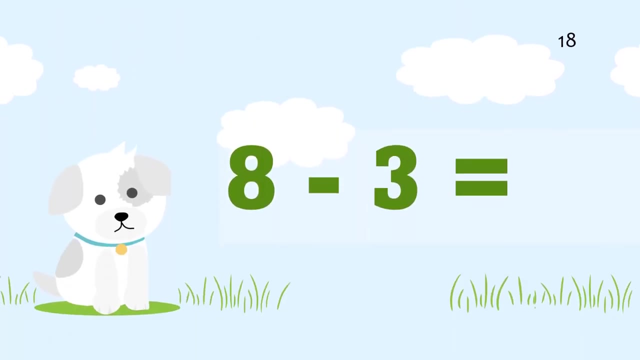 Pour a large bowl of water and finish it. This is my favorite time to play with the cat. She is so cute. It's so cute that you can't stop laughing. She is good at playing with cats. I think she will be fine. 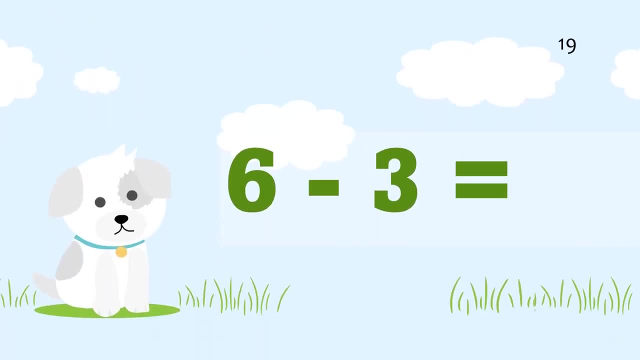 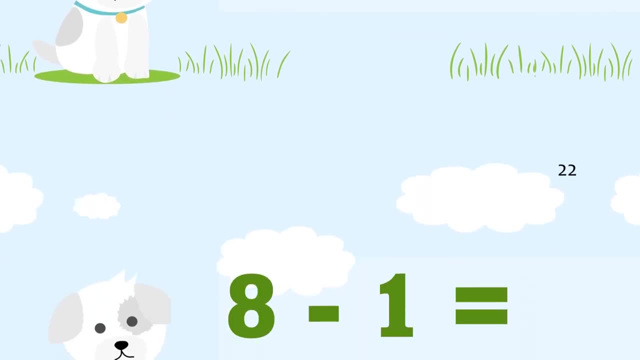 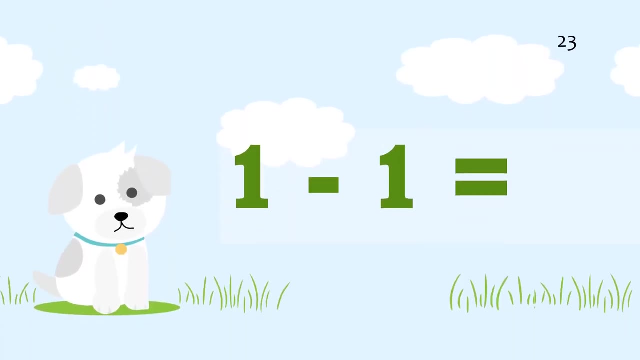 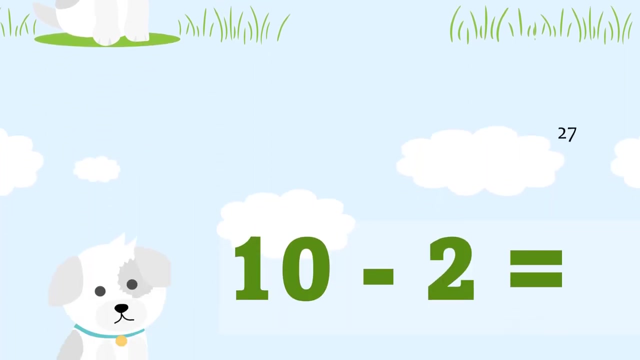 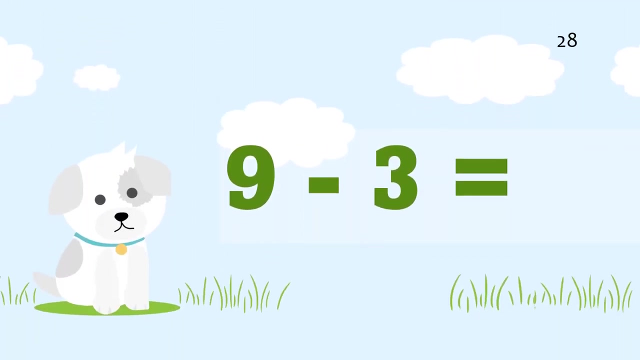 I'll take care of you. Salt, Black pepper, Black pepper, Boiled egg, Egg, Egg, Boiled egg. I can't help but laugh because I'm tired, I'm tired, I can't help it, but I'm tired, I'm tired, I'm tired. 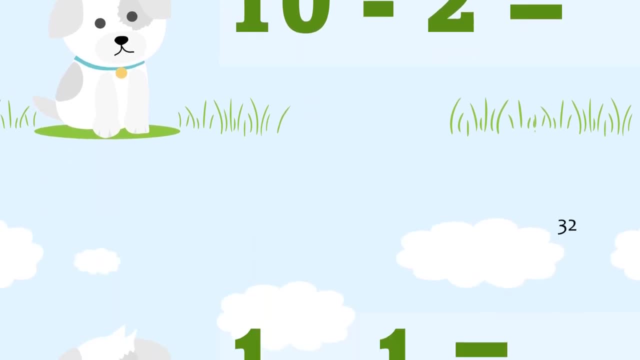 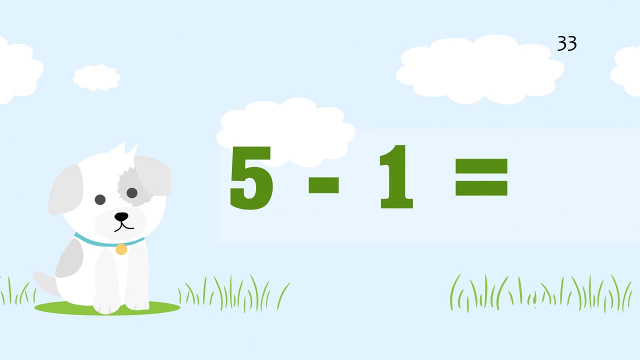 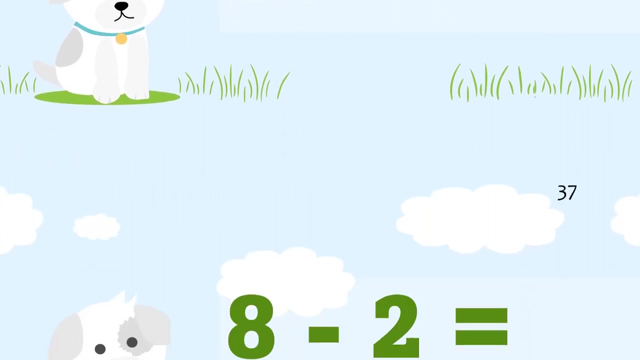 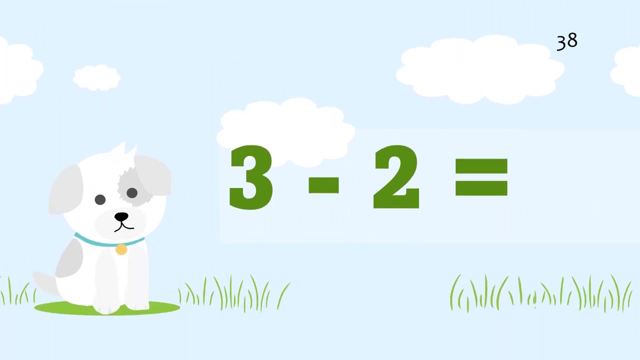 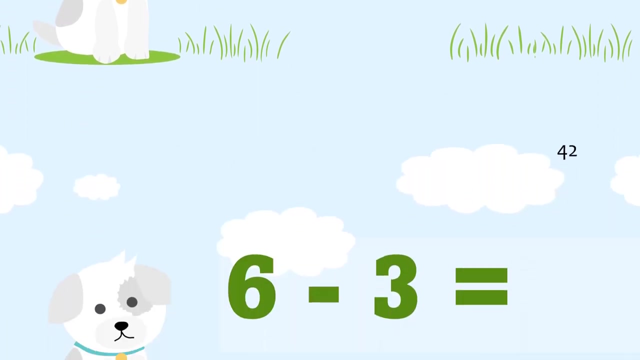 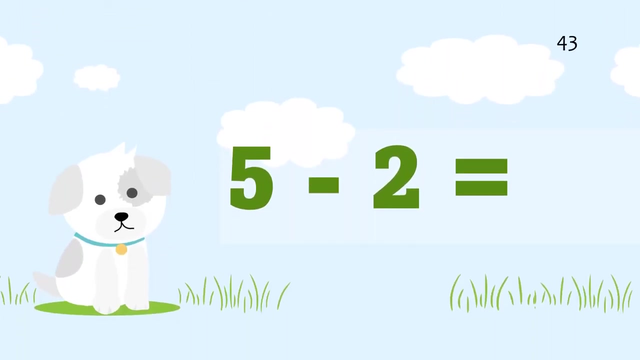 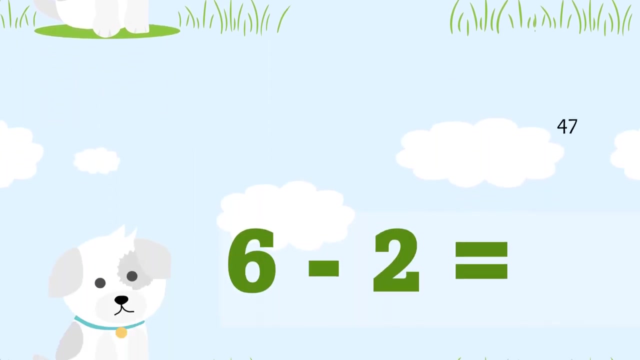 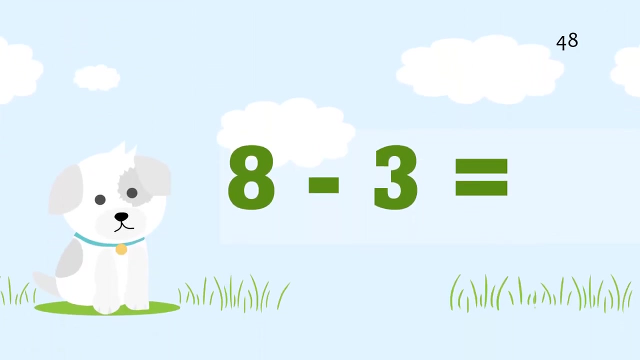 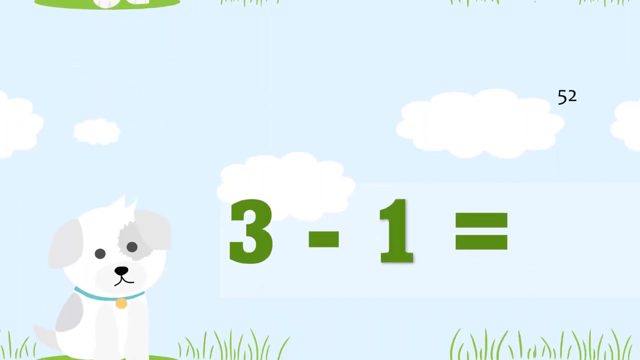 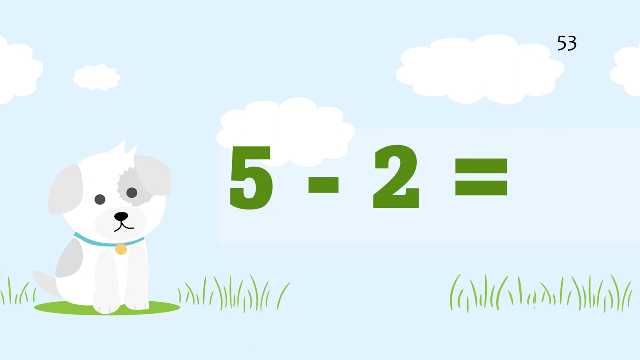 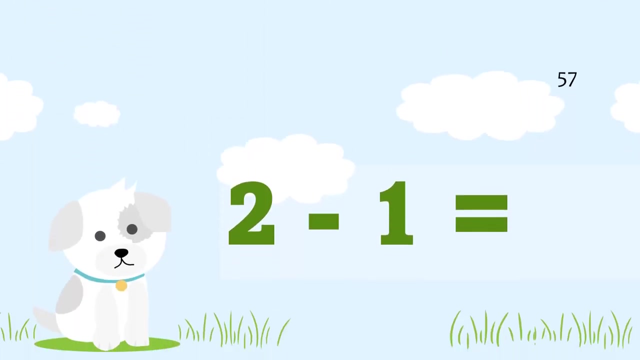 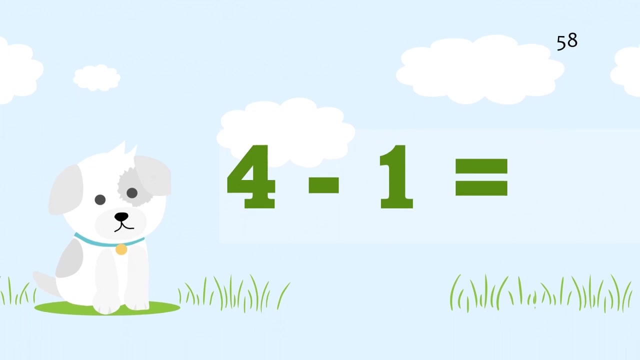 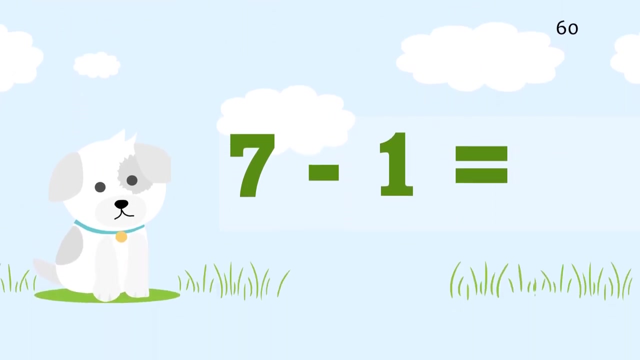 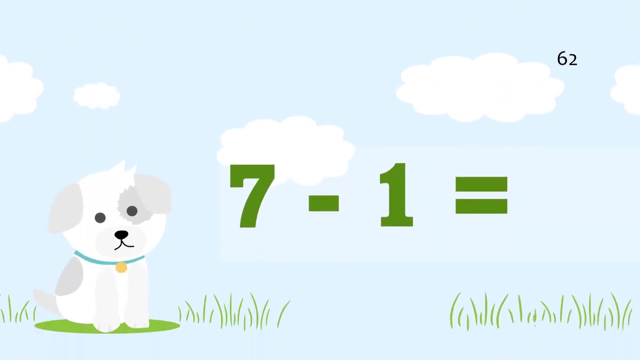 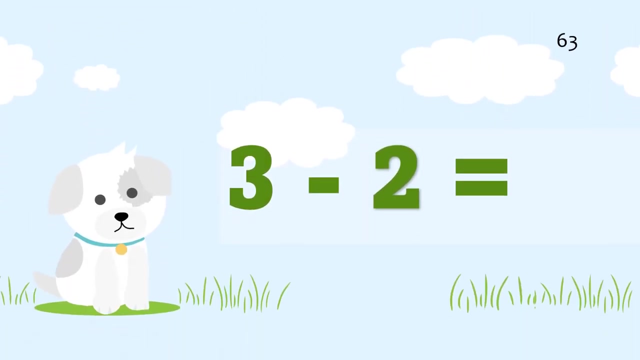 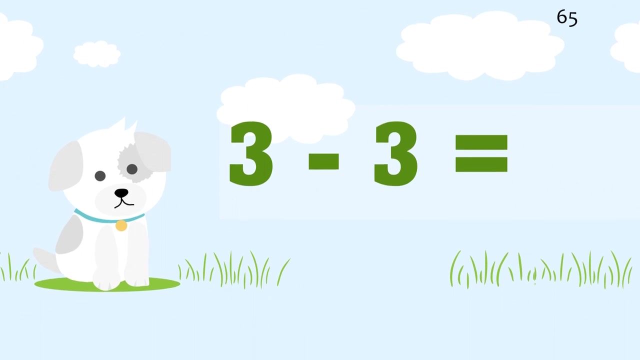 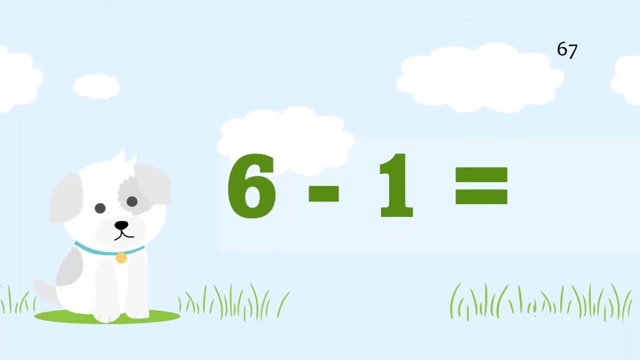 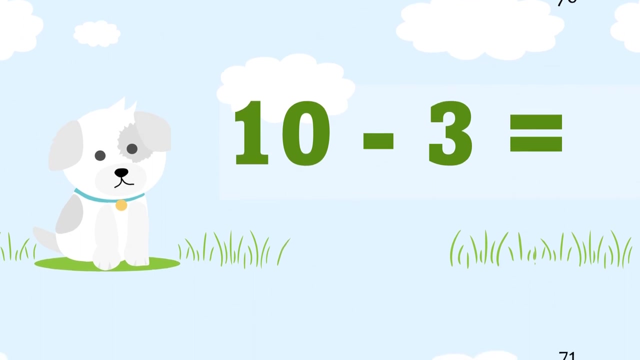 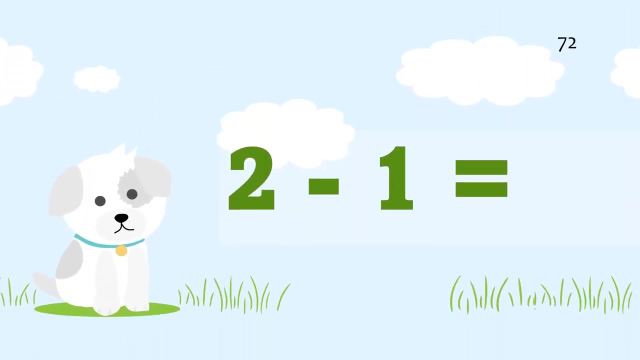 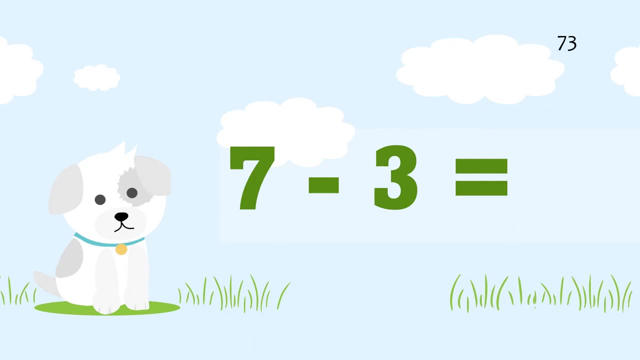 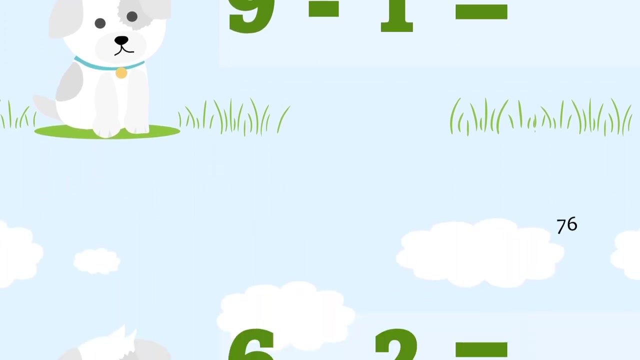 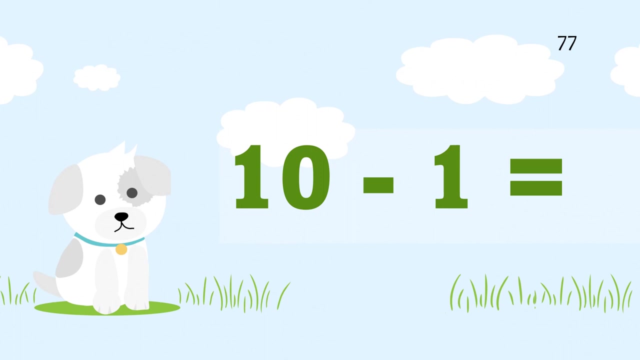 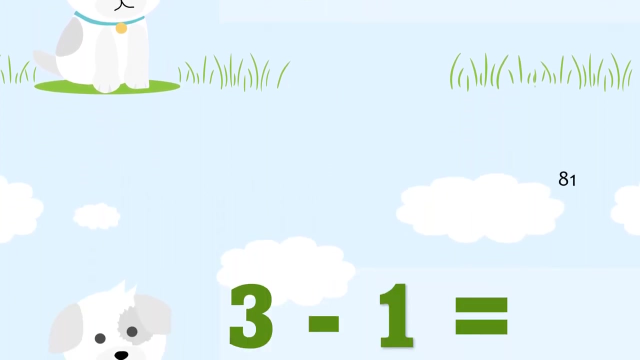 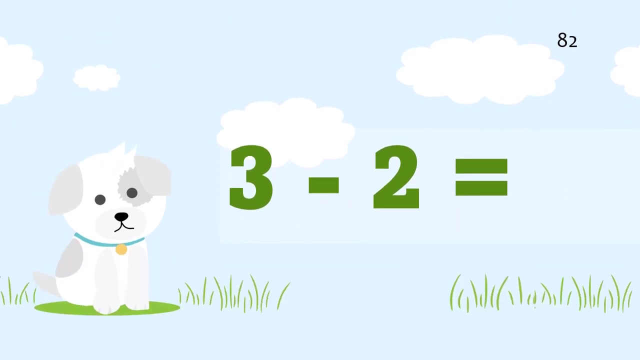 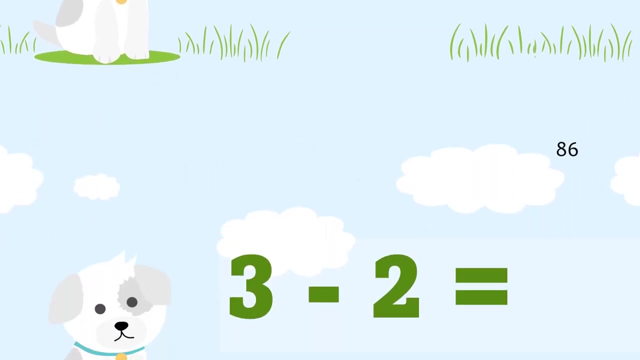 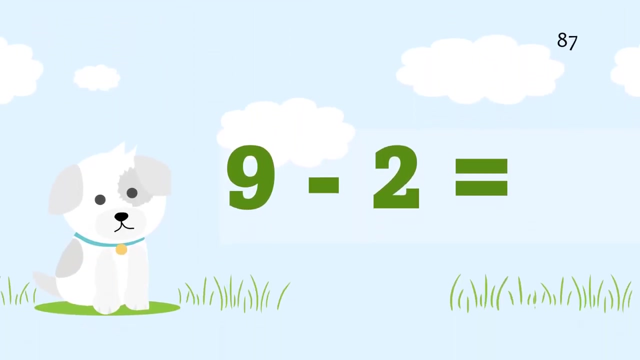 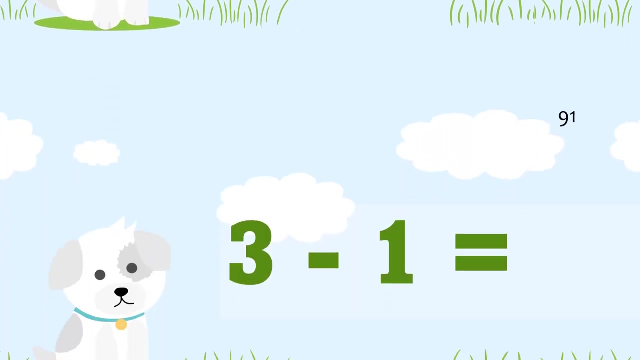 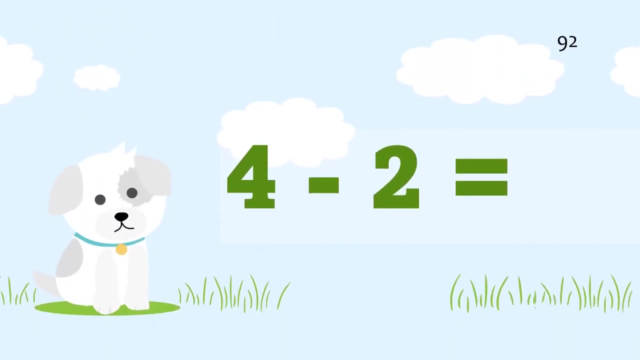 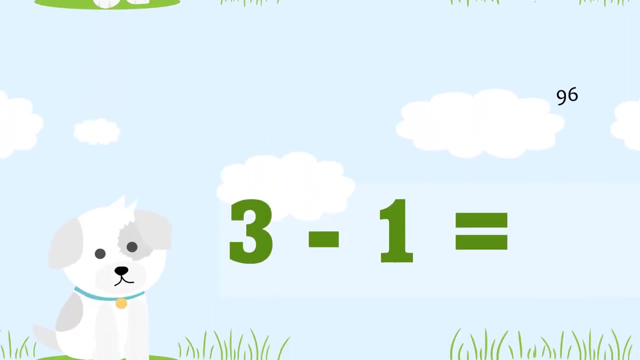 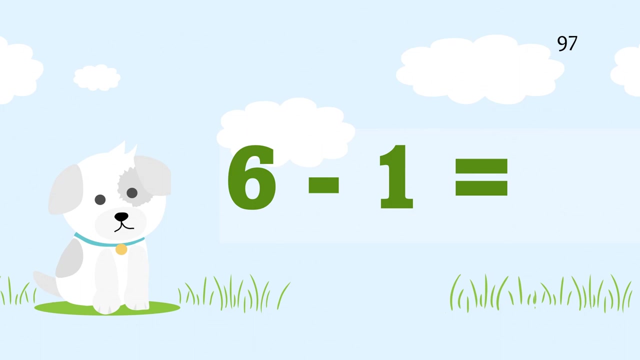 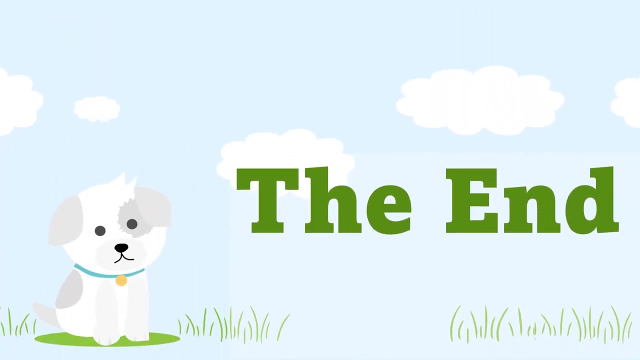 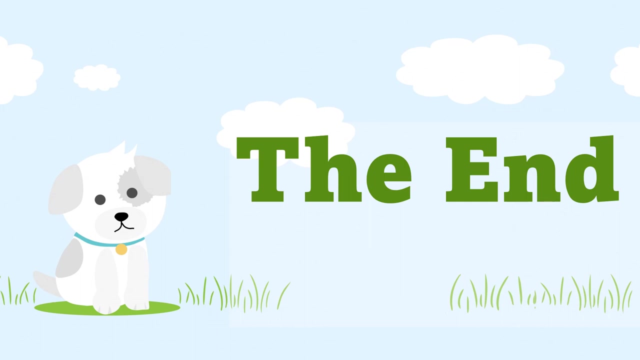 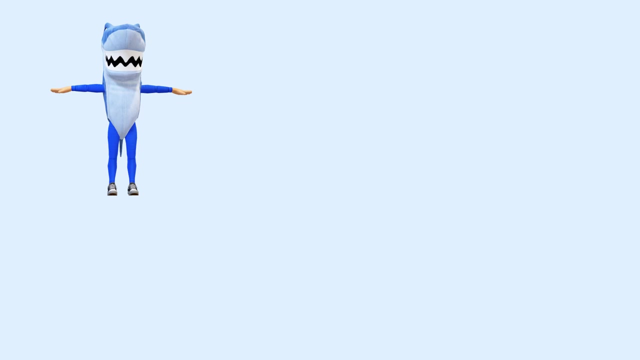